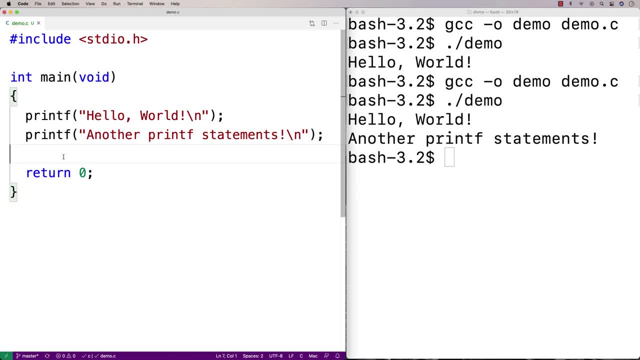 a large problem into a set of smaller problems and that sort of divide and conquer approach. that's a big thing in computing because if you think about a very large program- let's say it's- you know tens of thousands of line of code. if you wrote an entire main function that was 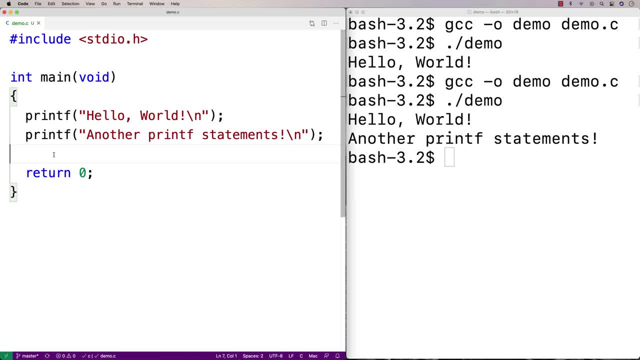 tens of thousands of lines of code. that's going to be difficult to understand and read because it's not really broken down into a set of more kind of comprehensible, smaller sub problems. So functions allow us to break our program down into a nice kind of logical set of sub problems. 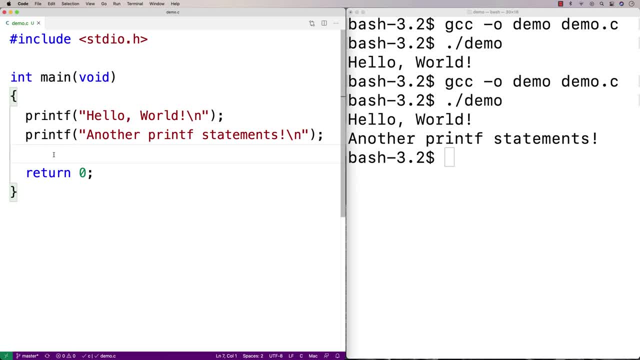 that might be utilizing each other. we might have functions calling other functions. we might have functions that utilize several of other functions, and that's okay. So that's another reason why we like functions is that they allow us to break our program down in a modular way. that's going to be more sensical, that's going to be more readable. 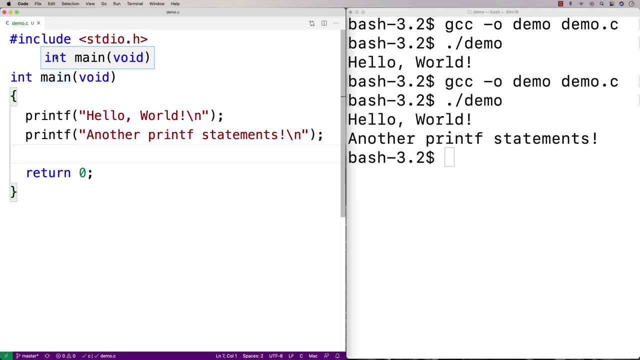 more understandable for others. Let's actually make a function here. I'm going to say here, int add, and I'm going to say int a, int b. then I'm going to say int result is equal to a plus b. then I'm going to say here, return. 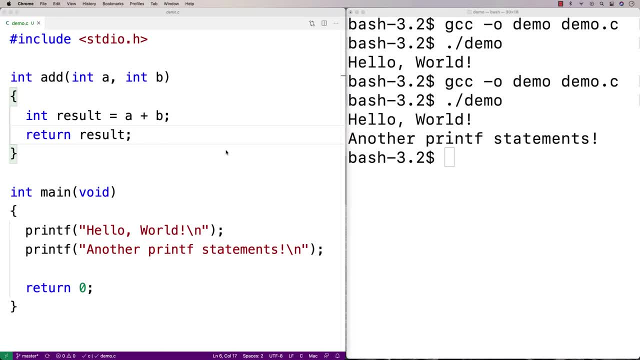 result. So, even though this is a small example, it actually contains all the key pieces of a function. so this here is what's called the function header and this here is what's called the function body, and these make the function definition. Now, what's going on here is that we're giving a name to the 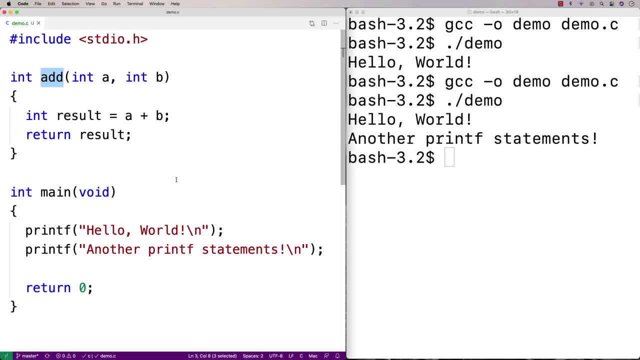 function. the name of the function is add and that's what we would use. if we want to call the function, we would use add to call it. so we would say like add, and we would then have to give something here. so add is the name of the function, this here, this int, here, that's the return value. 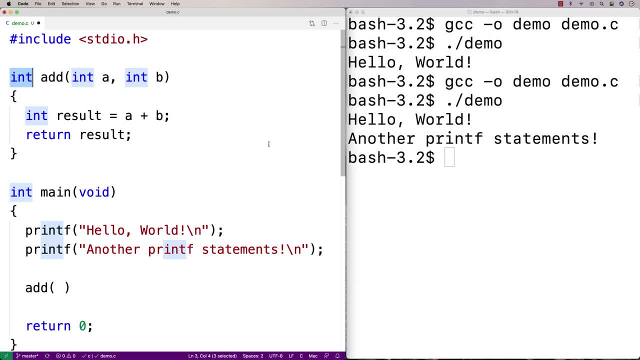 and this is basically telling the C compiler that this function is going to return an int value. Now, this here is what we're going to do. We're going to say int a and comma, int b. these are the parameters of the function. So we're telling C that when this function is called, we expect to provide it with 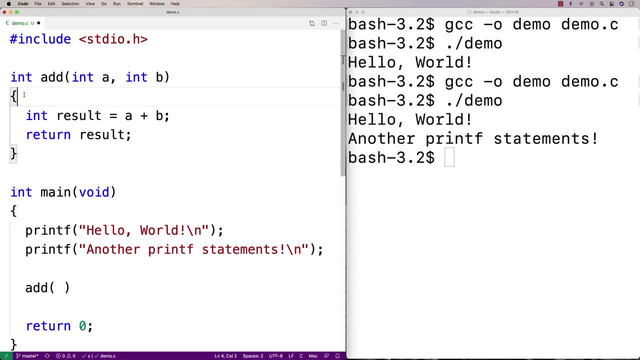 two integer values. We expect there to be two integer values provided And then inside the function body here, this is where we're going to execute the code, this is where we're going to actually perform some work. And so then we say int result- we can make a variable here- and we say: enter the value here. 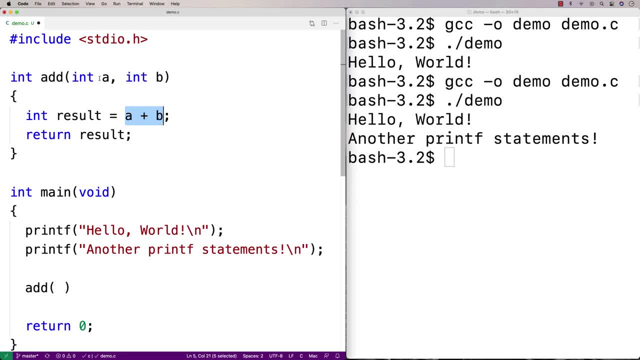 result is equal to a plus b. we add the two numbers together that are going to be provided to this function and we store the value in result, and then we return the result. so the return result, this is the return statement. now, functions don't always have to have a return, but they often do. and what? 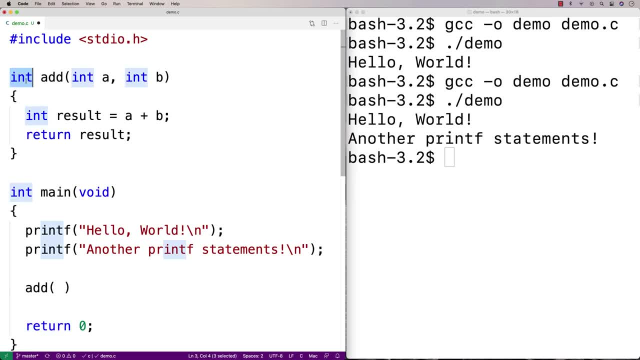 the return statement does, is it actually returns a value of this type. so it actually is going to return a value of this type here, and that's how the function is going to actually finish- is is that it's going to, you know, return the result, and then the function is done so here. if i were to say like: 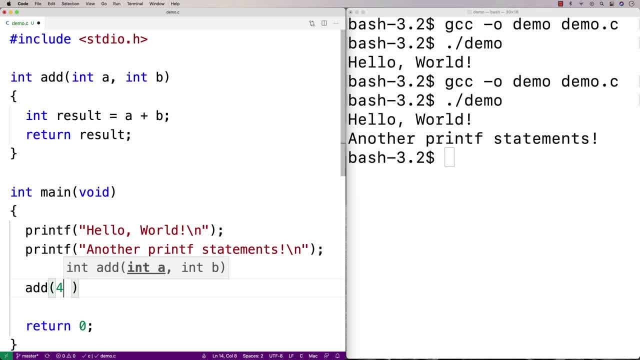 add, and i were to say four, five, or we'll say yeah, four, five here, and then i'll say maybe here i'll say int and i'll say maybe output is equal to add four, five, and then i'm going to say print f and i'll say output percent d and we'll, we'll just 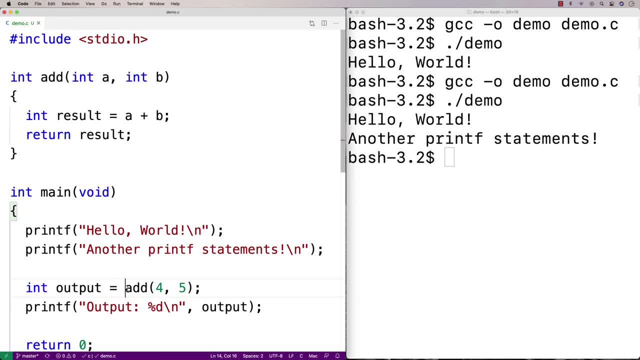 print out the output. so what's going on here is that we're calling the add function, and when we call the add function, we're providing with two arguments, four and five. and what's going to happen is is that a is going to be set to four, b is going to be set to five, then the body of 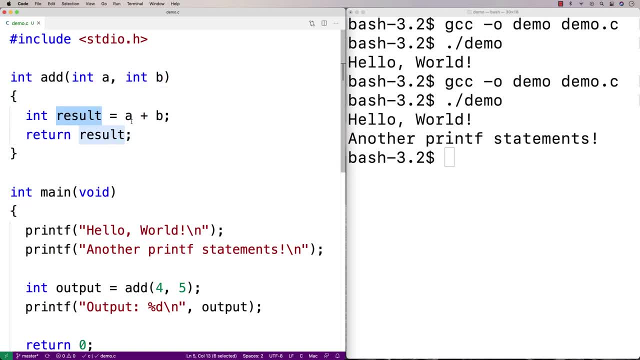 the function is going to run and we're going to create a variable result that is going to, you know, add four and five together and then result is going to be nine. then we return nine. when we return nine, it's kind of like a of like if we replaced add with the return value. So it's like if we did this, It's like if nine. 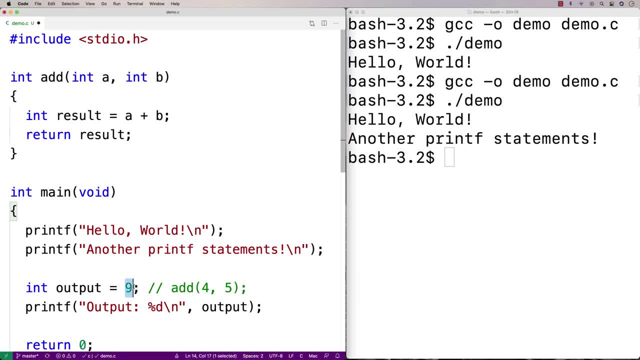 just appeared here and we just returned nine at this point. So nine is going to be the value that output is set to. So add is going to return a value And when it does, it's almost as if, like, you replaced this call to add with the value. It's almost like that. So when we say here, add, 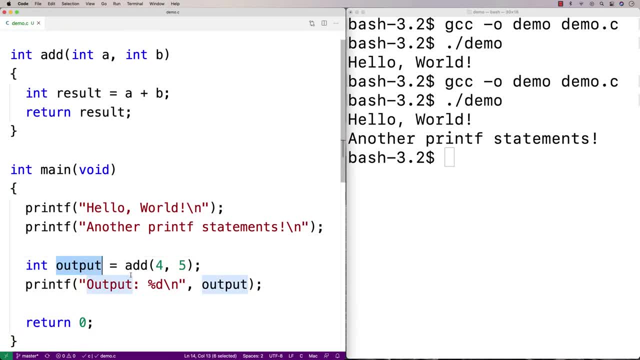 four, five. we're going to get nine back and we're going to set output equal to that value And then we're going to print out the output. So we'll just run this here, And I think I'm going to do is I'm. 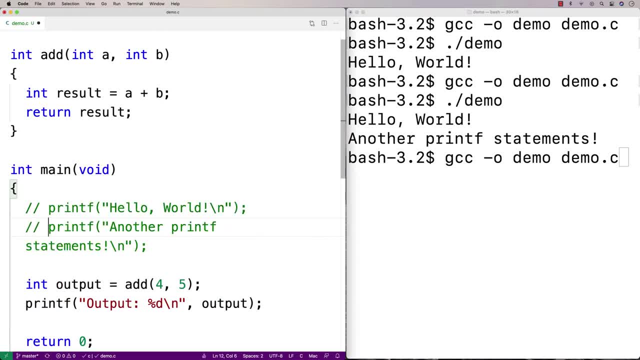 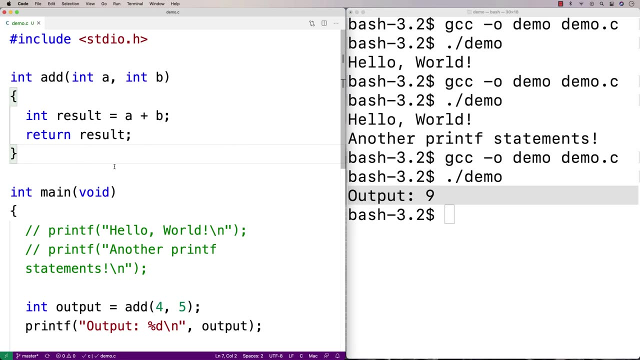 just going to comment out these because I don't think I really need these anymore here. And then I'm going to say here GCC to compile it, and we'll run it again and I get output nine. So that is a basic function there. And now a couple of things about this. One is we actually have the function? 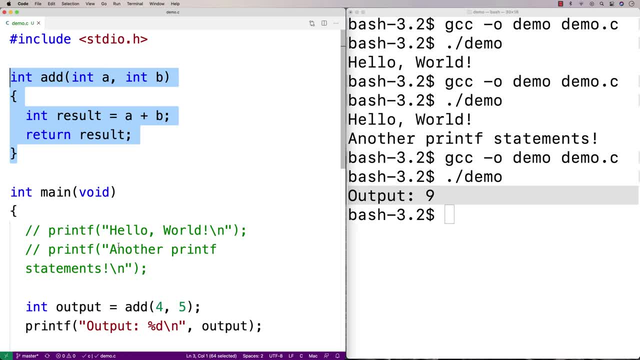 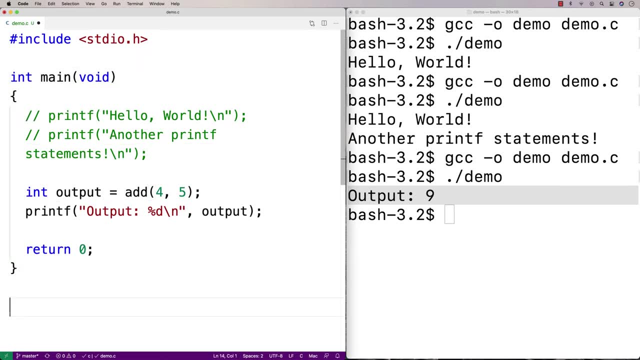 defined above main And we did that for a particular reason. So if I were to take this, so I'm going to cut it and I'm going to paste it below the main- If I were to take this and paste it below the main and then try to compile my program, we're going to find it's not going to. 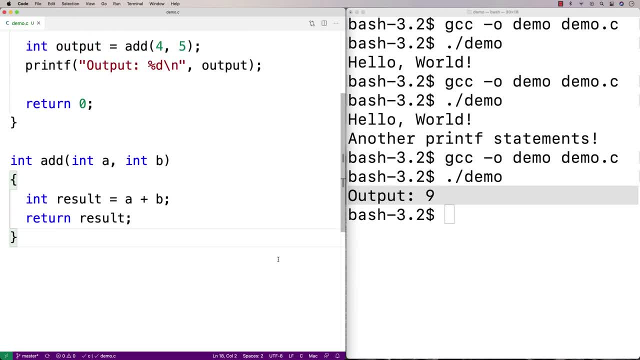 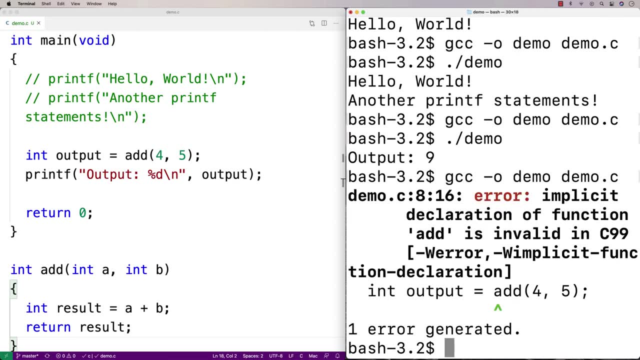 like this. We're going to find that the compiler is not going to like this. The compiler is going to complain about this. So we'll give this a shot. here We'll say: GCC, dash out, demo, demo, dot C, And the compiler here says error. implicit declaration of function add is invalid in C99.. 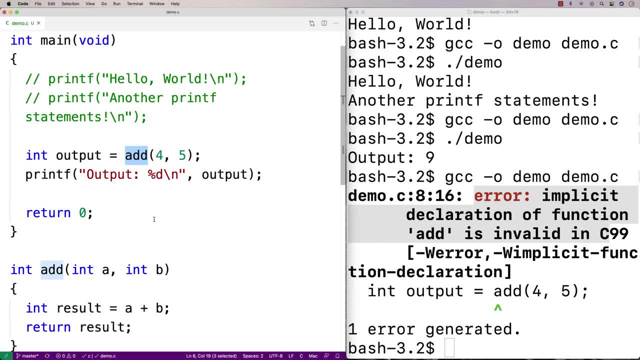 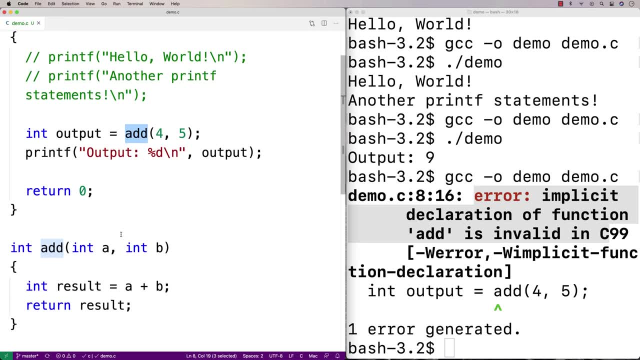 And basically what it's telling us is I don't know what this is. Implicit declaration means like where is this coming from, basically? And so it's telling us like I don't know what this is. So the problem is is that the way that C programs are compiled, when you call a function, the compiler 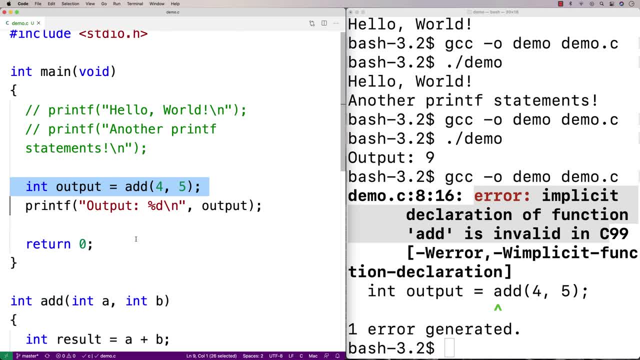 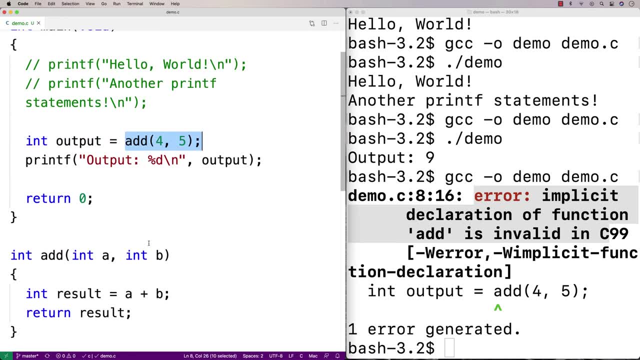 has to be aware of the function at that point. It needs to be at least aware that it exists. It can be defined later, but it needs to be at least aware that it exists. So oftentimes what you'll see in a C program is that the main function will be at the top of the file and the 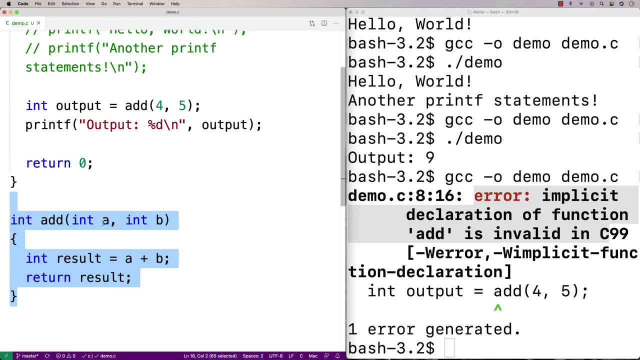 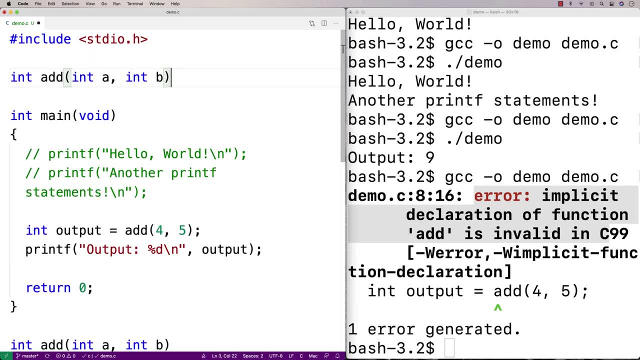 functions that main might use are defined below it. But what you'll see is this: We'll copy and paste this function header here and we're going to put it up here and put a semicolon there. What this now becomes is what's called a function declaration. So we're not defining the function. 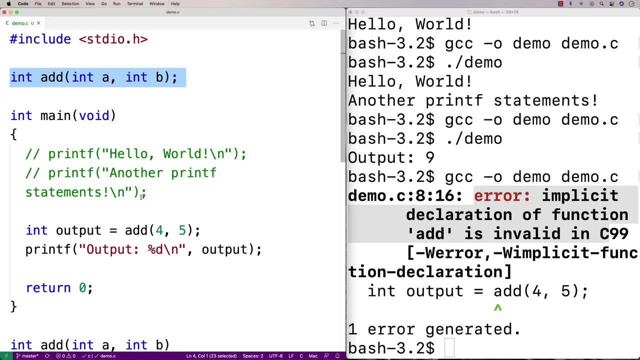 here, but we're telling C, we're telling the C compiler, really, I should say- that we want to have a function called add. It's going to return an integer and it's going to accept two integers as arguments, And we're telling that to the C compiler by putting it here. So that way, when 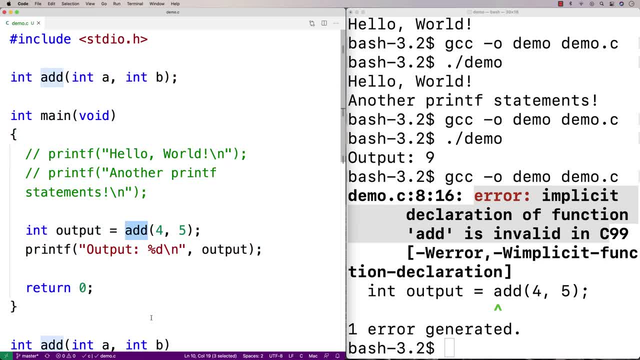 the main function gets compiled and the compiler sees: add. here it says: okay, I don't know what the definition of this function is yet, but I do know that it's been declared. I know that it's going to exist, So sure you can go ahead and use it. And then down here, now we've actually 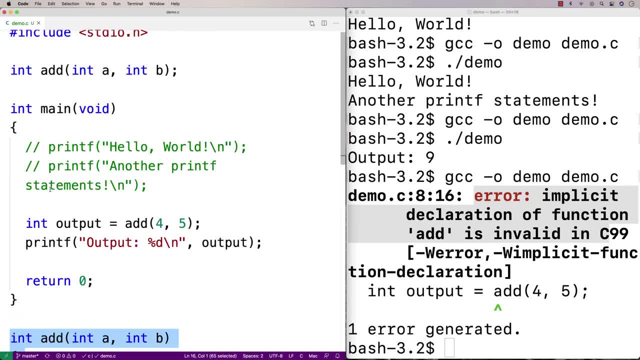 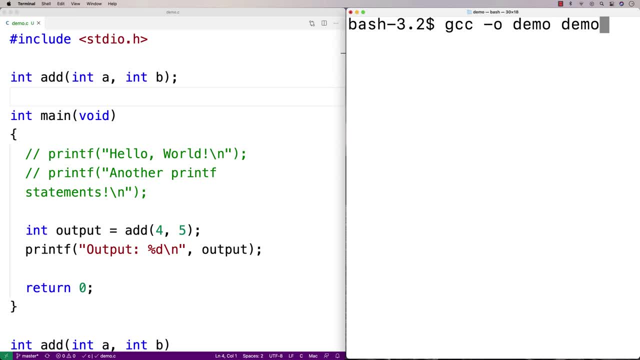 provided the function definition. So we call this the definition, And then what you can do is you can you know? we'll just clear this here Now. if we compile it here, it'll actually work And we get back to an output of nine. So one of the reasons why you 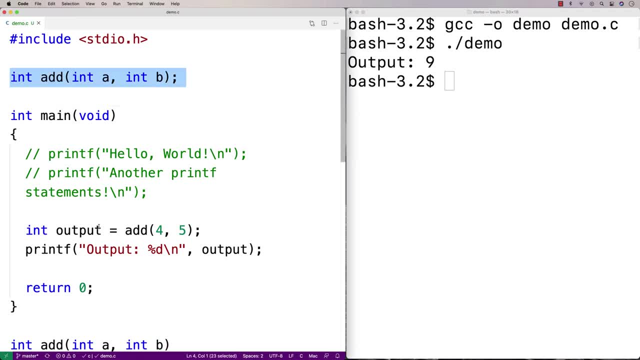 might want to do this is that if we had a bunch of function definitions up here, then the main function, which is pretty important because it's the starting point of the execution of our program, would be buried below a bunch of function definitions. We can also have multiple function. 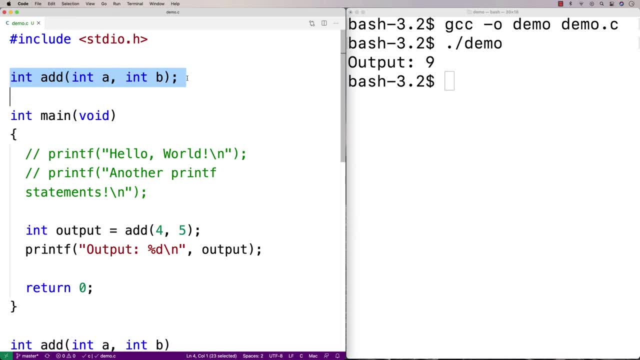 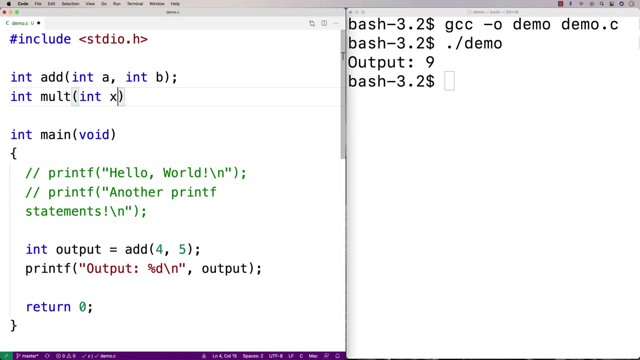 definitions and we can. we can have functions that call, you know, the other functions we've defined. So let's make another function. We'll call this one int, We'll call it mult, And mult is going to take in two parameters. We're going to say int x and 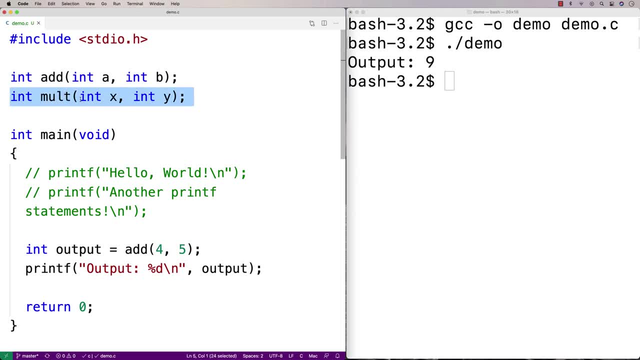 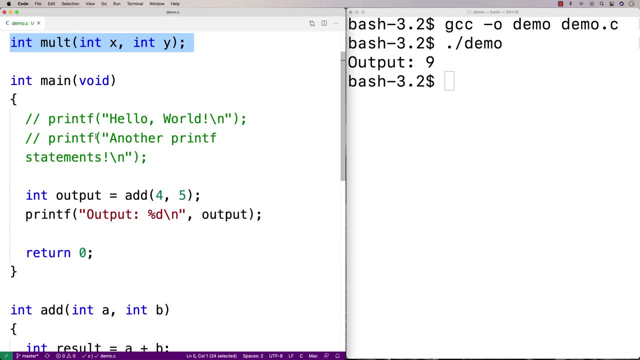 int, y And mult is actually going to be another function, but it's going to use our add function And we're going to actually implement a very inefficient multiplication function. So we're going to make a multiplication function here and it's going to take in two values, x and y, to 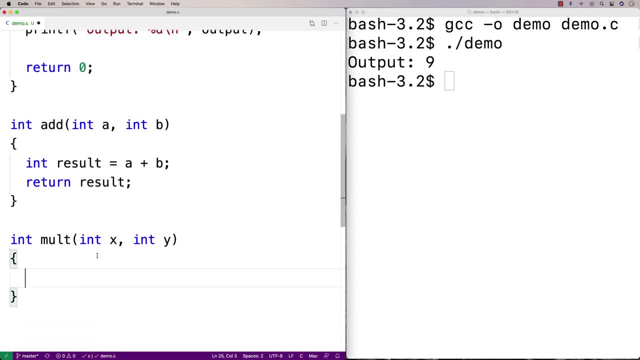 multiply And we're going to assume that they're both positive integers and what we're going to do to perform the multiplication is that we're going to add y to zero x times. so we're going to say here: int result is equal to zero. and i'm going to say here: 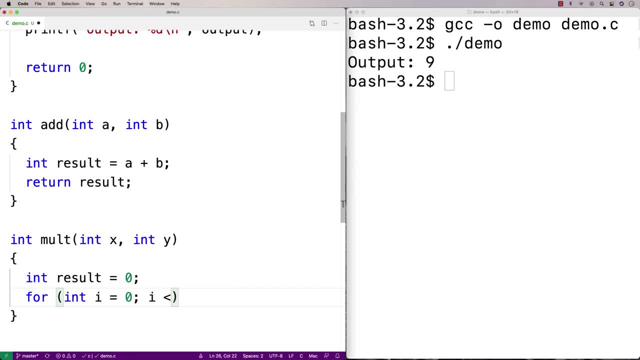 for int. i is equal to zero, i is less than, and i'll say x, and i'll say i plus, plus here, and we'll add to this result y, and we're going to add y to the result x times and then we'll return the result. 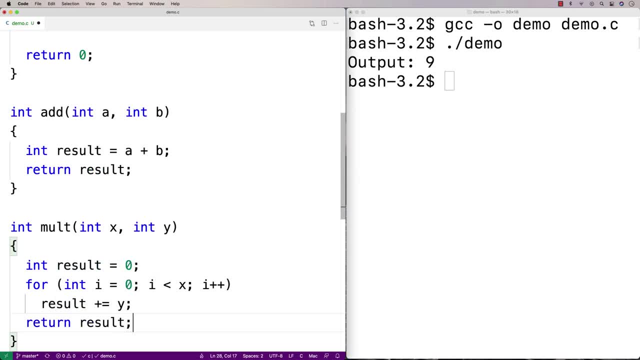 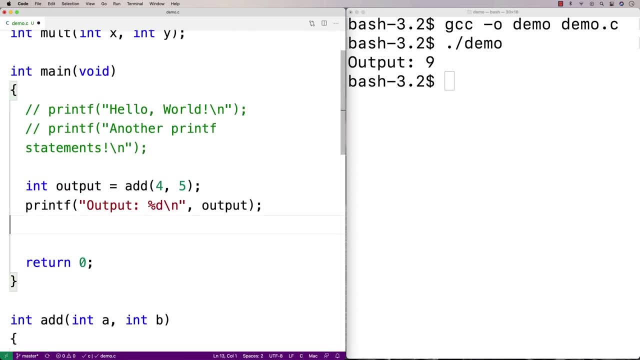 so this is going to be a super inefficient multiplication function because it's doing a bunch of additions to perform multiplication. so we'll give this a shot. here we'll say print f and we'll say mult output, percent d, and i'll say here: mult output. and now i'm going to say here: 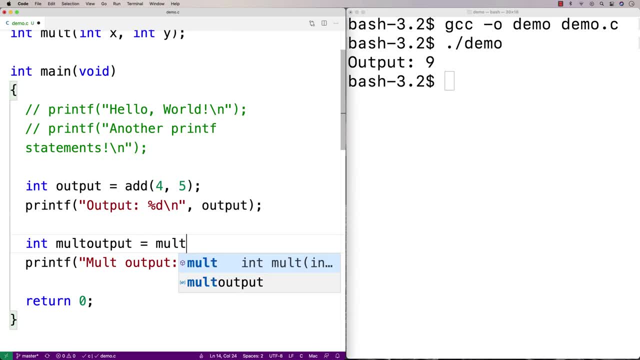 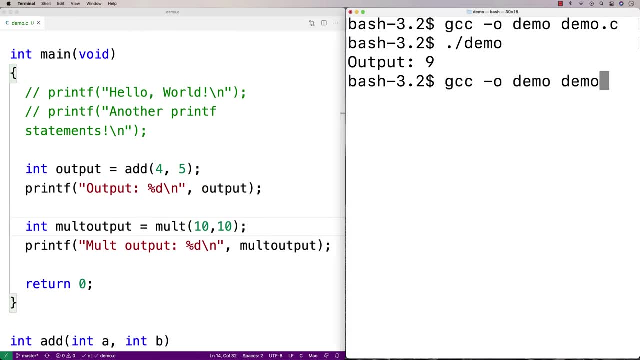 here int mult output is equal to. we'll say: multiply 10 and 10, because that should be 100 and we'll give this a try. so now we've defined another function here and i can run this here and i get multiplication output of 100. that seems correct. 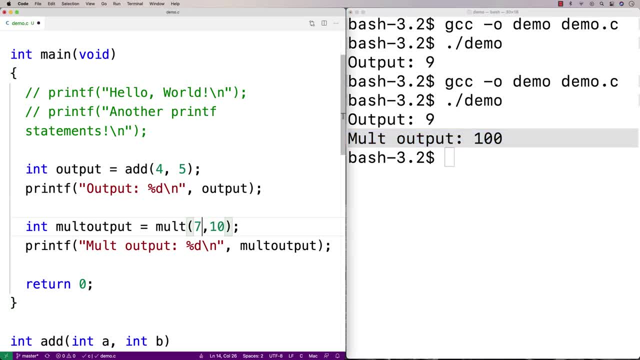 let's try something a little trickier. we'll try like nine and, oh sorry, nine and seven, and we'll just give this a shot, just to give our function. another test here: we got 63, so So our multiplication is working and we've defined another function here. 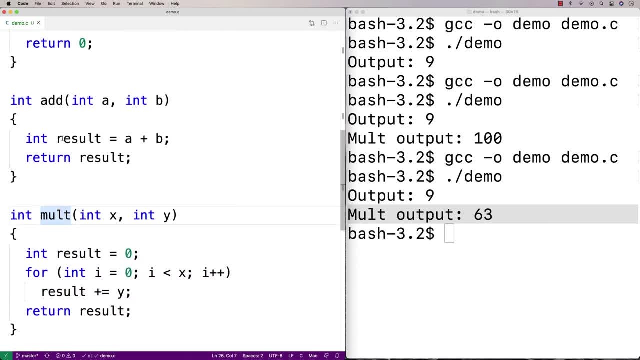 Now what we could also do is we could have this multiplication function, use our add function, So functions we've defined can call other functions we've defined. So I could say, instead of result plus equals y, I could say: result is equal to add result, and then I'll say y. 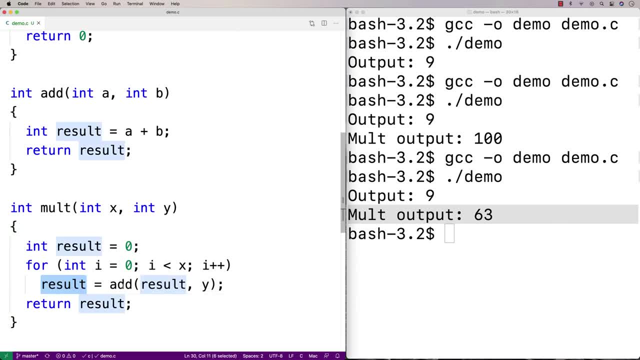 So basically I'm saying: set result equal to the addition of whatever result is currently and y, And so if I run this here, I still get 63. So I recompiled it and ran it and I still got 63. And it's because I'm just changing it to use our add function now and I've got a function here that's using another function. 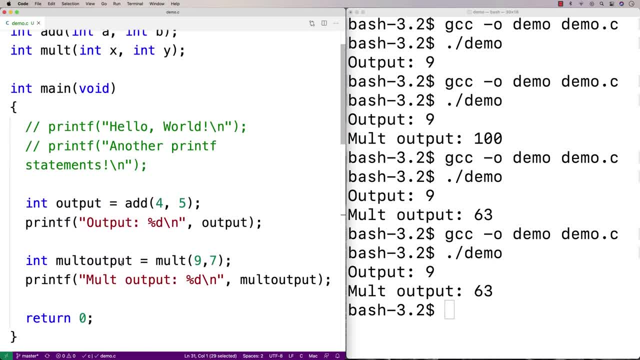 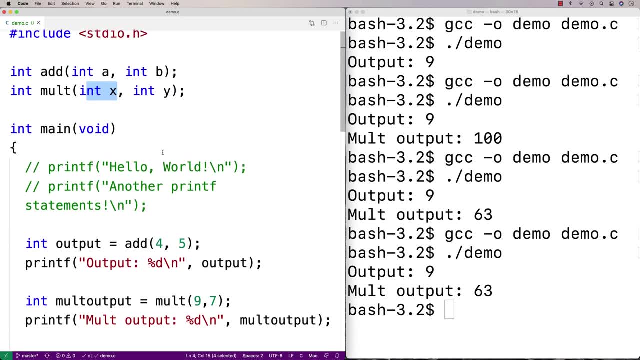 So now, one other thing about functions that we really want to make sure we understand is: what's the relationship between the add function and the add function, What's the relationship between these values here and these variables here? Because what's going on here, if you look at it, is I'm giving specific values here. 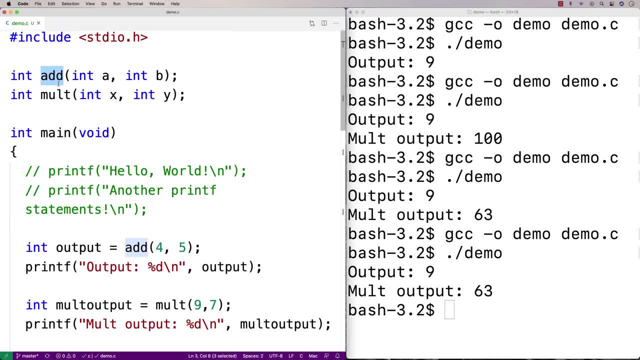 Like here I'm giving 4 and 5, and we call add and int a is going to be set to 4, int b is going to be set to 5.. In this function here I give it the values 9 and 7.. 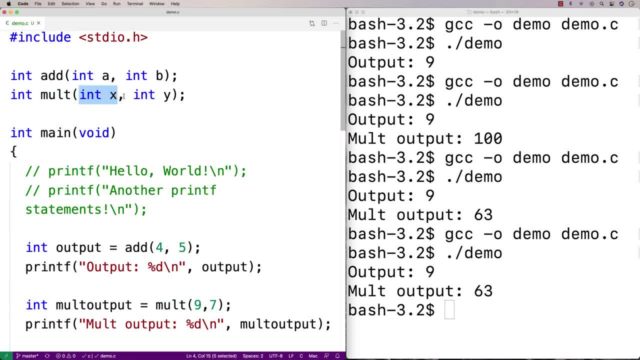 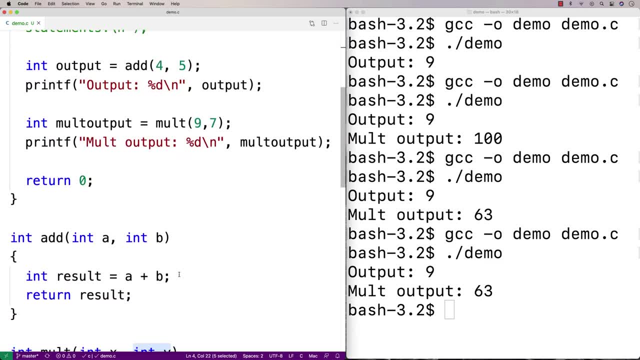 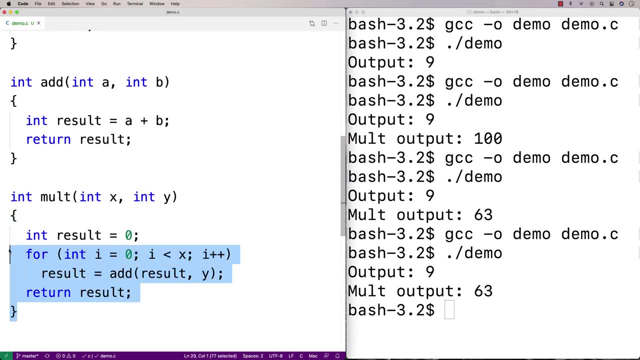 Multiplication is going to be called and when it's called, x is going to be set to 9, and y is going to be set to 7.. So there's a difference between arguments and parameters. Parameters are these, Parameters are the variables, and these variables are going to be local to this function. 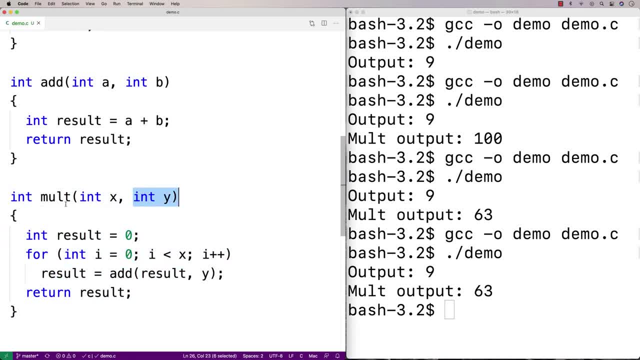 So int x and int y. they don't actually exist outside of this function. We call them local variables because they're local to this function. here And when we pass in an argument like this, this is a particular value. These are specific values. 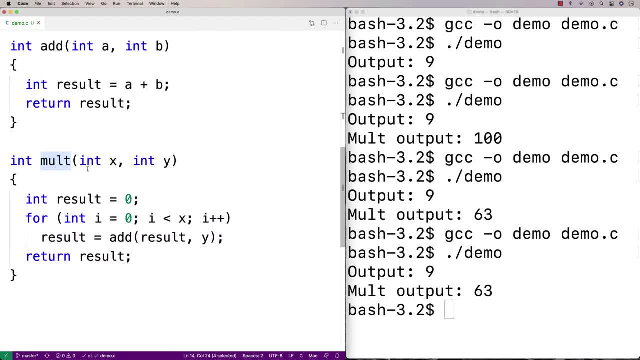 And when the function is called, what's going to happen is it's like we've created a variable x and set it equal to 7. And we've created a variable y and set it equal to 9.. So that's one big thing to understand is that when you call a function, you're basically setting these, you're initializing these parameters to a particular value. 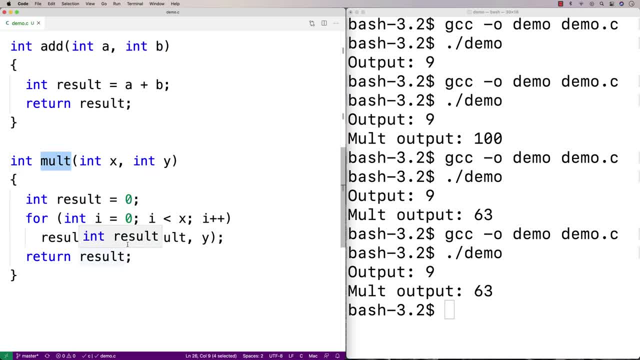 So, for example, in this mult function here, when we call add and we say result and y, we're not really giving it like the variable result and the variable y. What we're giving add is we're calling add with whatever value result is currently, which is initially going to be 0. 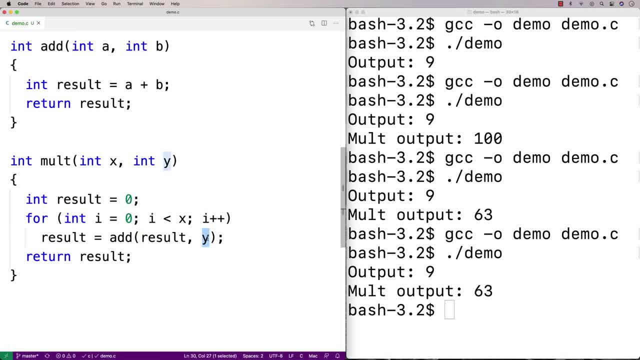 0. And we're going to call it with whatever value. y is currently So like, add is just going to get some number for a and some number for b, And it's going to do some work with them and then return another number, which is going to be, you know the result of this function. call here. 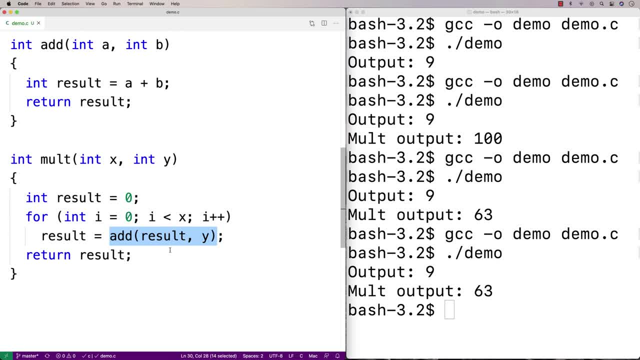 And that's it, And so we don't really like there isn't really a relationship between results and a and y and b beyond that, And so that's just something to make sure you understand is that the functions are being called with a value. 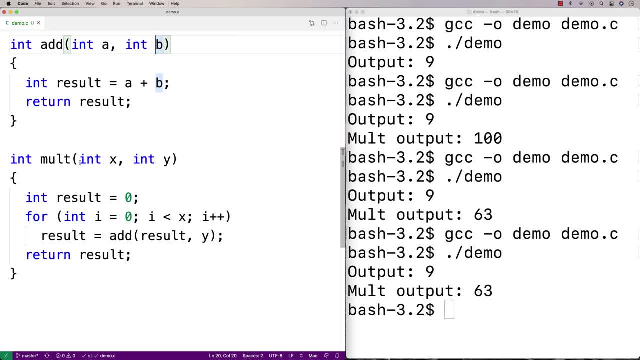 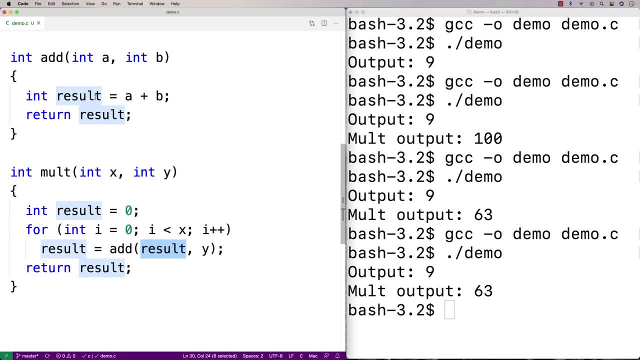 As the, as the arguments and the parameters. here these variables are set to those values And that's the only relationship there. It's not like result is somehow like the same result is in this function here or being used by this function here beyond its value, being used when the function is called as an argument. 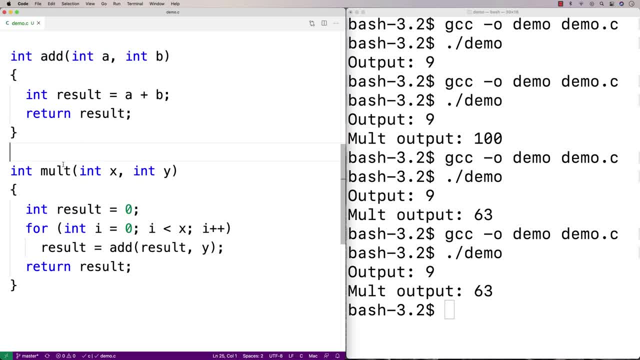 So that's one thing about functions. Now, another thing about functions is variables like this, like int, result. These are also local to the function. So this variable here, result, It only exists when this function is called And then that's it. 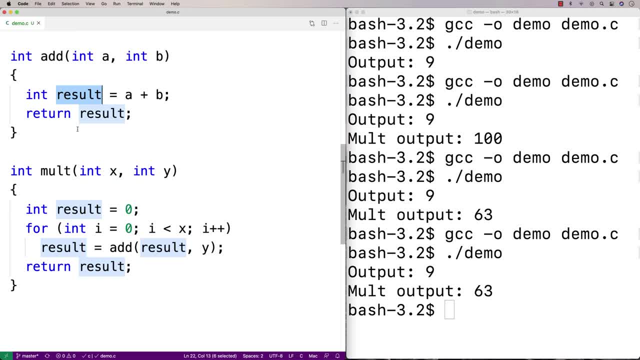 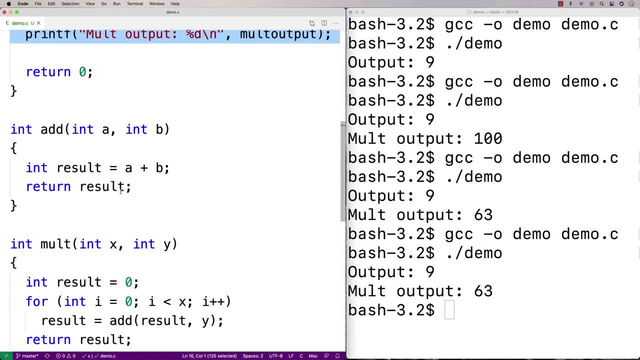 It's done, It no longer exists, And it's just. it's local to the function, So we can't use result outside of this function. It's not like we could use result in our main function. That's another important thing about functions.